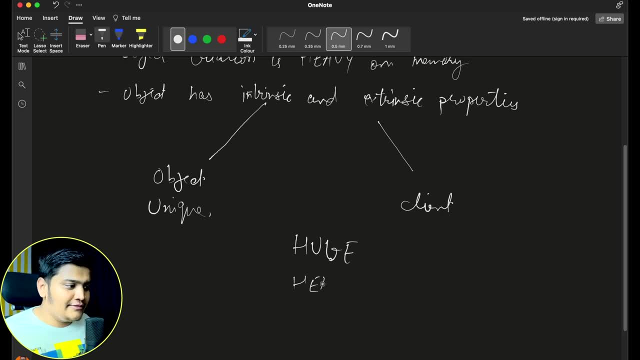 number of objects and the objects are also heavy, right? That's when we will be using the flyway design pattern. So suppose let's take the example where you have to create a lot of objects, right? So let's take the simple example where you are creating the 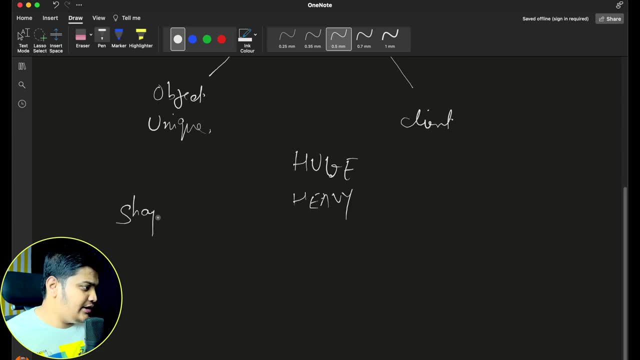 shapes, right? So suppose you have to create shapes And whenever you want to create a shape- suppose you have oval shapes, you have line, you have rectangle- okay, These are the different shapes that you have and whenever you want the object, what you. 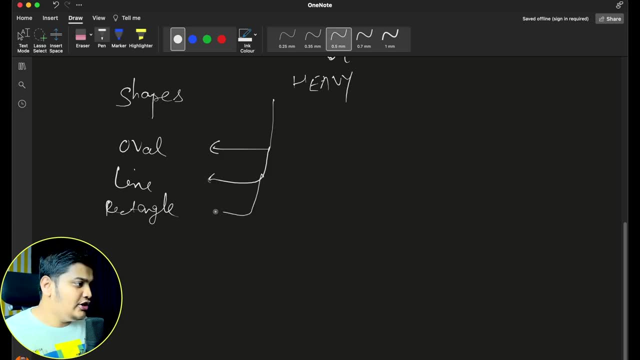 will do is you will call the constructor of these okay to create the objects. and whenever you will call the constructor, the new object will be created for it and you will get that particular object And suppose, for every object creation, for every object creation, suppose it is taking. 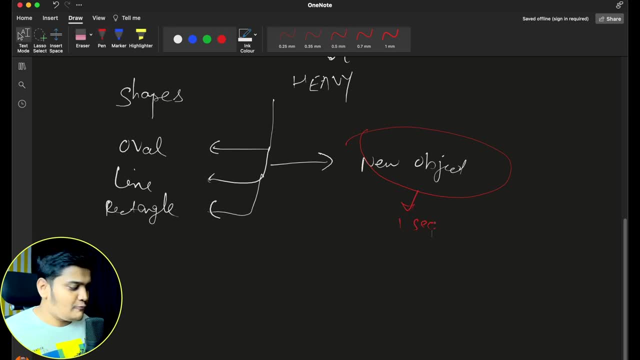 around one second. Okay, So it's taking one second to create the objects. So what will happen is like: whenever you will call that I want the object of an oval with all these like it should be filled, it should be not filled. it should be with this border. 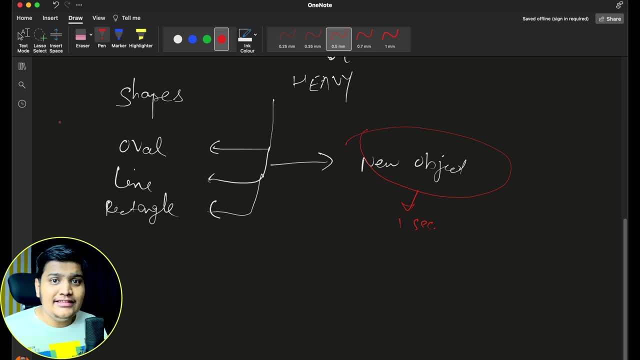 it should not be with this border, it should be dashed. whatever the properties are- and there might be some properties defined by the client as well- like: the oval should be drawn at this x and y direction. all those different things are there and the oval should be with this. 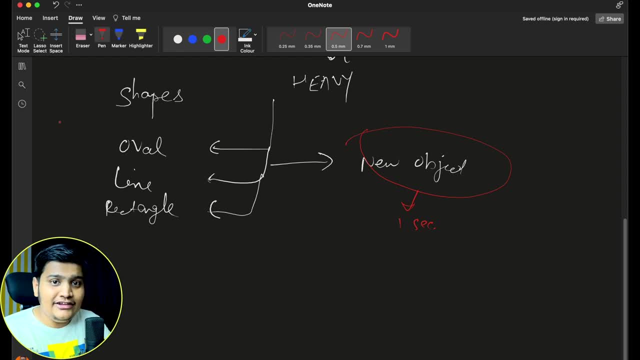 this much width and this much height. all these different properties will be set by the client. those are extrinsic, like what should be the fill, what should be border, all those who are intrinsic properties that can be directly used if there is a case and the object creation is taking. 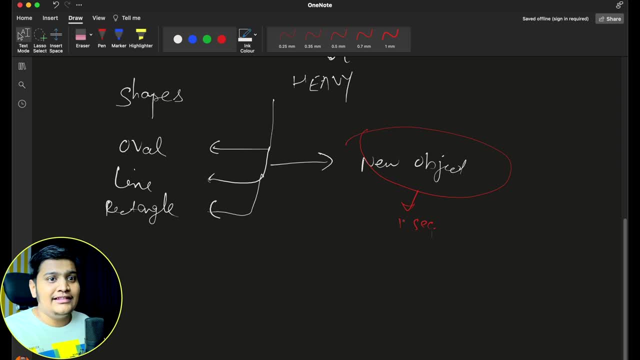 too much time. so for every object creation you will take that much time and the processing will be too slow, right? so it's very huge and heavy process as well. so to avoid the scenario, we will use the flyway design pattern in flyway design pattern. what we will do is we will have the 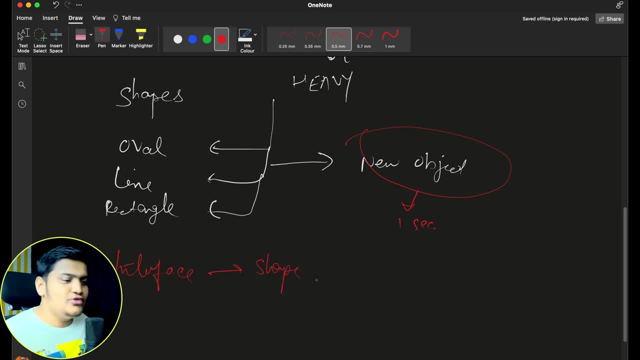 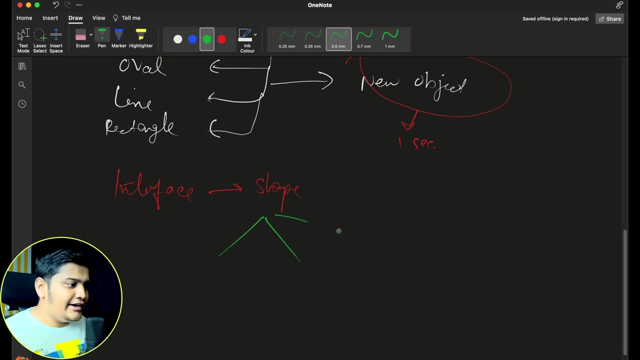 interface for shape. okay, let's use this example itself. we will have the interface for the shape and for this shape, different concrete classes are there. suppose: line is there, oval is there, rectangle is there? okay, now, based on this, concrete classes, all these concrete classes will have the intrinsic properties and 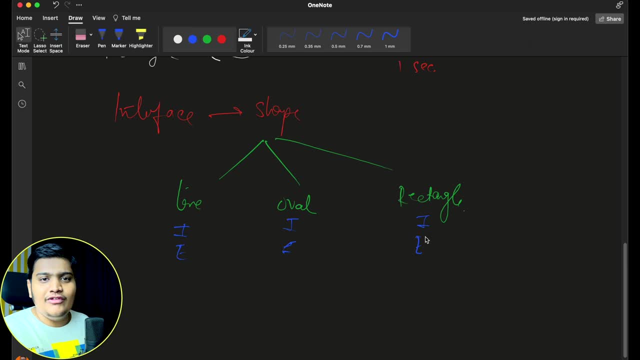 extrinsic properties. intrinsic properties and extrinsic properties: all will have different types of properties. i suppose line will not have any intrinsic properties. it will have extrinsic properties, like to which position the line should be drawn. oval like oval, should be filled or non filled. the border should be. 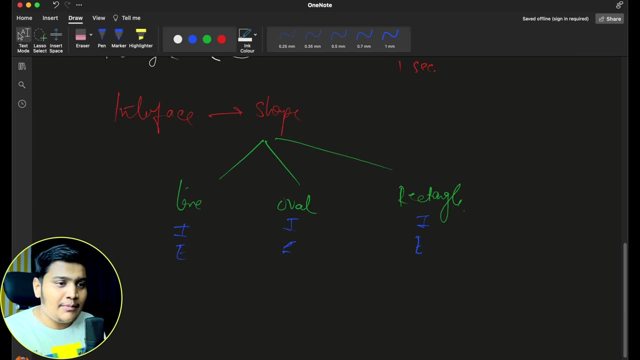 normal or dash border, that's. these are the different intrinsic properties. extrinsic properties will be like in which position this oval should be drawn. those are the extrinsic properties. okay, so you can see that there is a difference where we can identify the intrinsic and extrinsic. 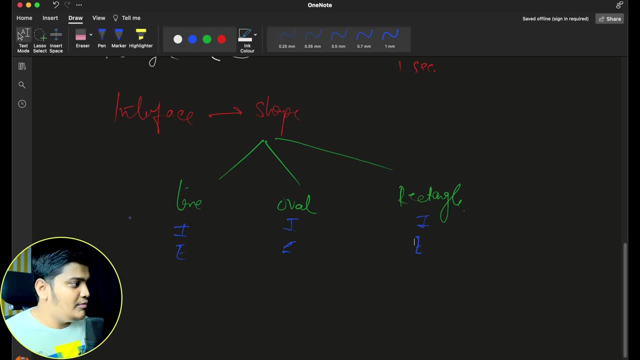 properties for each of the different shapes. now, for all of this, there will be a constructor as well, right to create the object, but directly we won't be using it. the client won't be directly using the constructor to get all the objects. what we'll do is we'll create a flyway factory. okay. 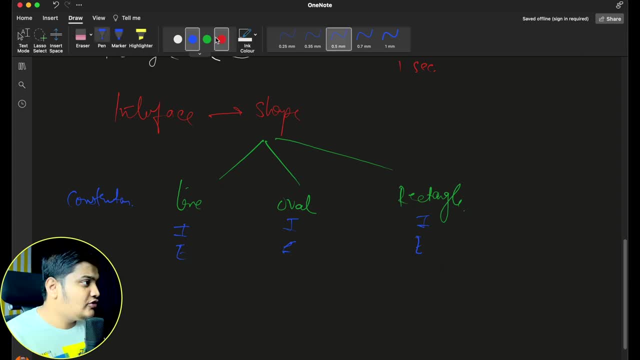 and from that factory itself the objects will be created. right? so what i'll do is i'll create a flyway factory and within this flyway factory, we will define what type of shape you need and, based on the type of the shape, what we will do is based on the type we pass. okay, based on the type we pass. 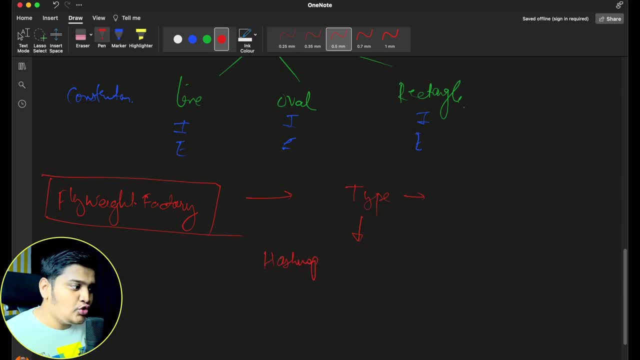 what we will do is we will have one hash map. what we will do is we will store all the different objects. we won't try to create each and every object every time. if the object is available within the map, we will use the same object. if not, we will create. 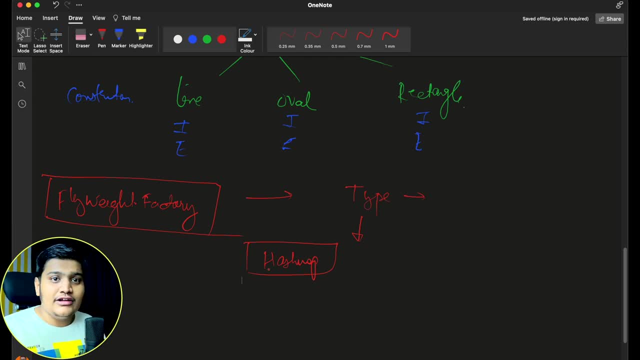 the same object. we will use the same object. if not, we will create the same object. if not, we will new object and we will store in the HashMap. So every time, what we are doing is we are not creating the object. so that means whatever the heavy lifting is there to create the object. 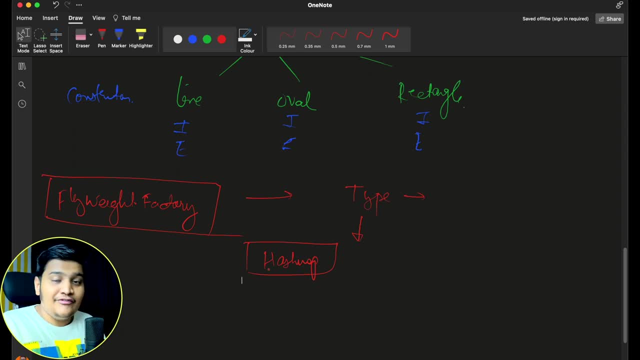 that we are minimizing. Whenever the object is created with the intrinsic values and we need the same object, we will just return it. Suppose the type of the object is: I want Oval, fieldOval. okay, That is one of the type. suppose I want Oval as non filled? okay, Suppose I. 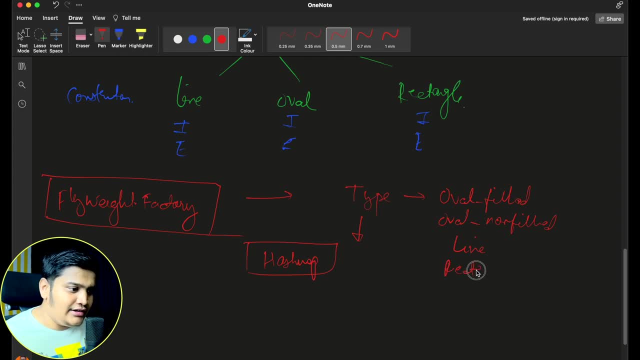 need a line. Suppose I need a rectangle as a field. okay, These are the different types of object. Now what will happen is based on the type defined here. okay, Within the map we will check if this particular type is available or not. If not, we will create a new Oval with. 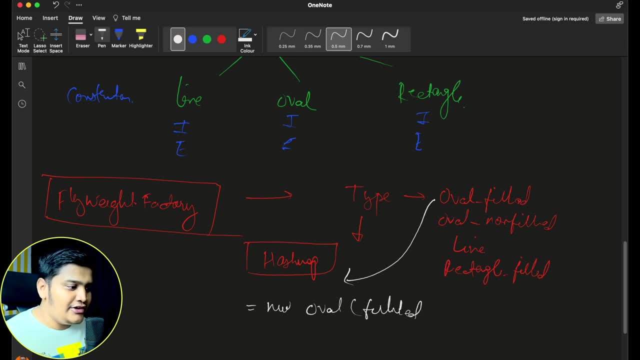 the type whatever is defined, that is filled with the intrinsic values, and we will create the object and we will store the same object in HashMap as well, And the next time, if the client is asking for the same Oval field, we will check in the HashMap and we will return. 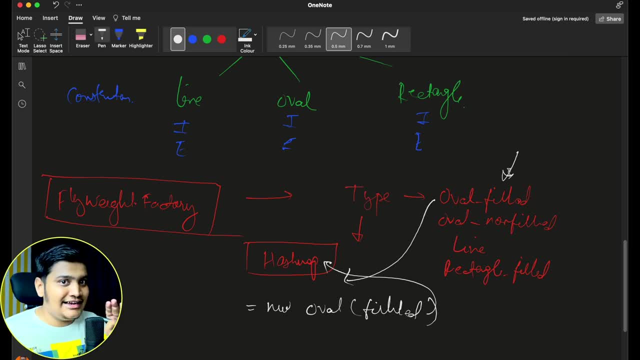 the same object. So, whatever the time is getting consumed in creating the object, that is been neglected now and all the intrinsic values are already set within the object and those objects are already available, So directly we can utilize those okay. So that's the general. 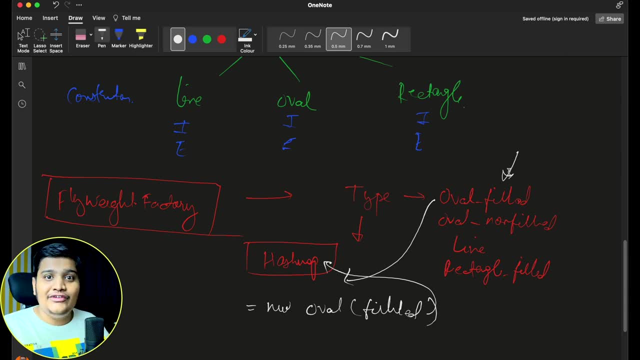 idea behind the flyway design pattern and the flyway factory, which will help us to utilize the already existing object with the intrinsic values, and the extrinsic values will be directly been set by the client, which is calling this factory okay. So this was the overall idea. 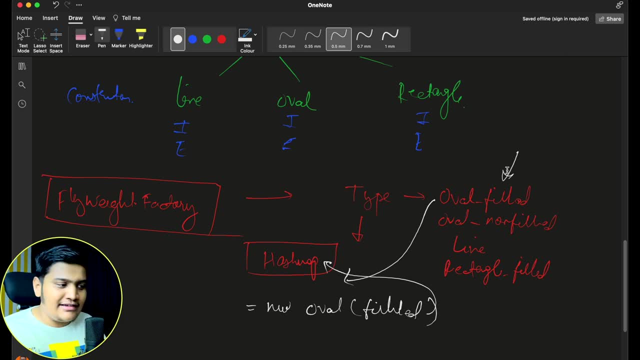 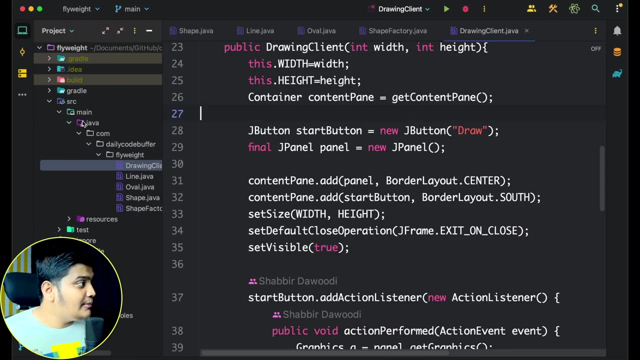 about the flyway design. Let's see with the example as well. So let's see the same example that we have used here, that is, the shape one. So if I go to the code here, okay, you can see that I have created the flyway project and within that we have different classes. So let's first go here. 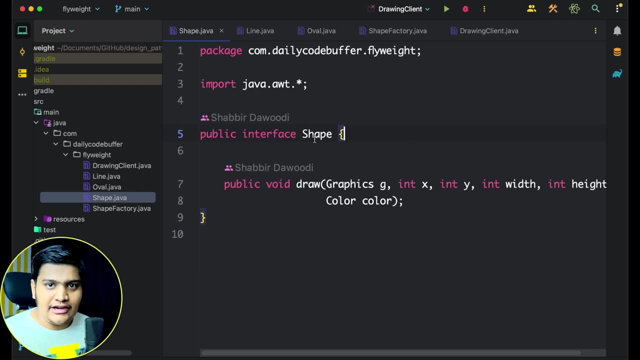 I have the shape interface here. you can see that this is a shape interface and within this interface we have one method, that is draw. and what draw is doing is it's taking the graphics. it is taking x and y, position, width and height and the color of the shape. 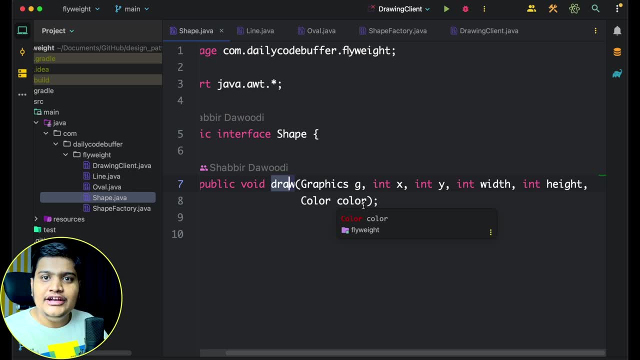 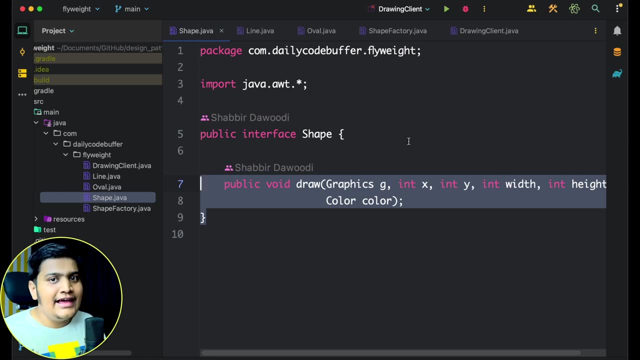 that you want to draw. This is a simple method defined, and all the different shape that we are going to create that will implement this draw method, and all the different shape will have the different intrinsic and extrinsic values. So let's go towards the line, okay. 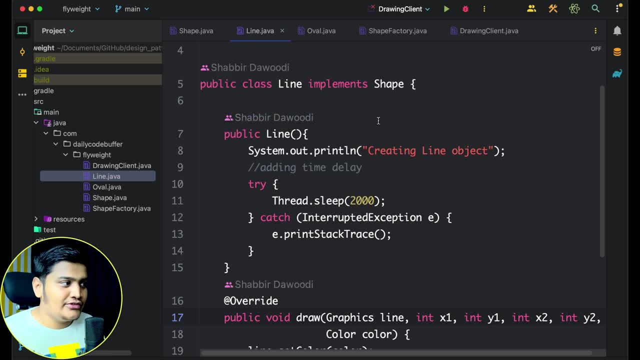 So line is implementing shape, but line doesn't have any intrinsic values. So what it is doing it it is just having a constructor here and what we are doing is we are just printing that, creating a line, and I am just adding a thread. dot. sleep of two seconds. Why I am? 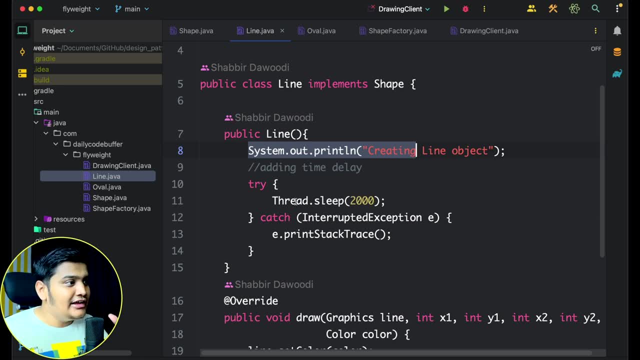 doing this is just to have the delay like just to mimic that the object creation for line is taking some time to create. So whenever I am creating the object first time, that time it there will be a delay, but next time, when I want to use the same thing, there won't be. 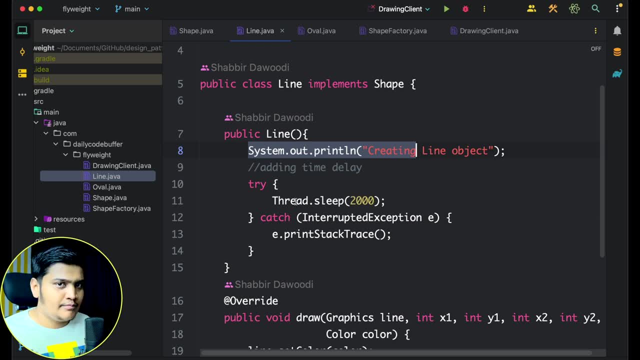 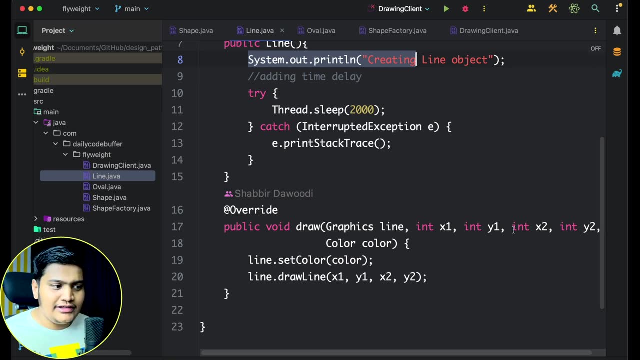 delay to mimic that, I am just using the thread dot sleep here. okay, So this is the constructor that I am using and there is a draw method as well, where I am taking the graphics line, all the xy positions and everything, and I am just setting the color and I am drawing. 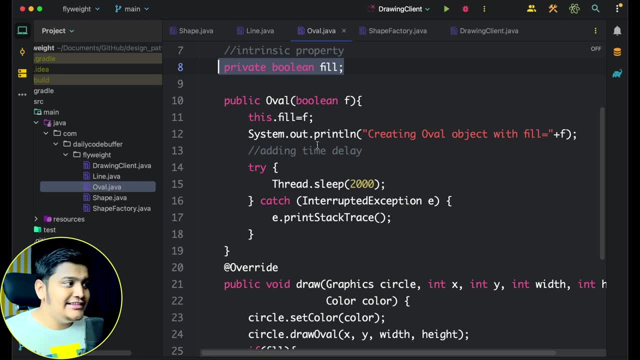 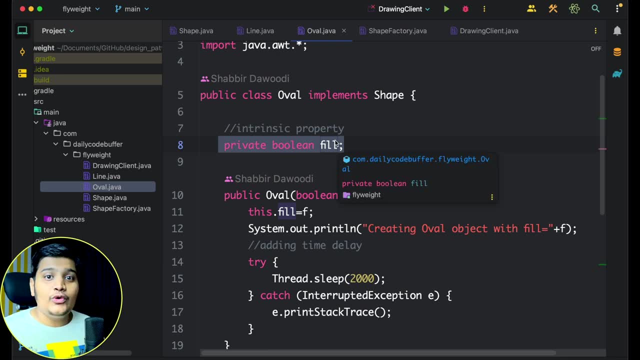 the line here. So this is a simple thing. okay, If I go to the oval here, you can see that for oval also, I am implementing the shape and for oval there is an intrinsic property that is fill. What is the fill type? do I want to fill or do I not want to fill the oval For same thing? 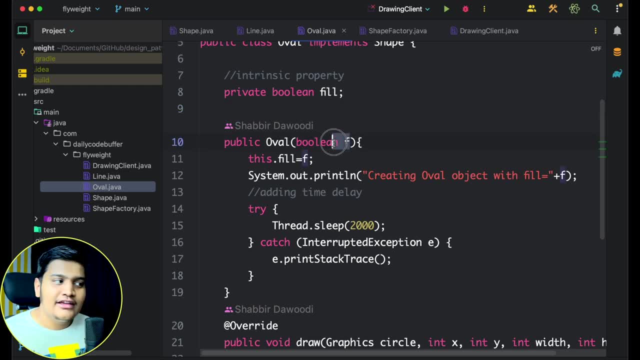 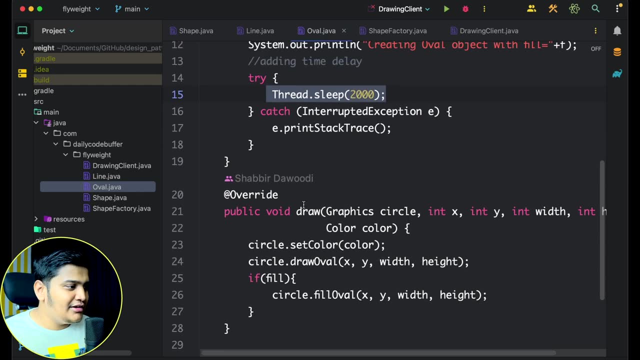 there is a constructor here and this constructor- you can see that I am taking the boolean f here that is, fill, true or not? and I am taking the thread dot sleep here to create the object. Similarly, I am just using the draw method to draw that oval. okay, Now for this. you can. 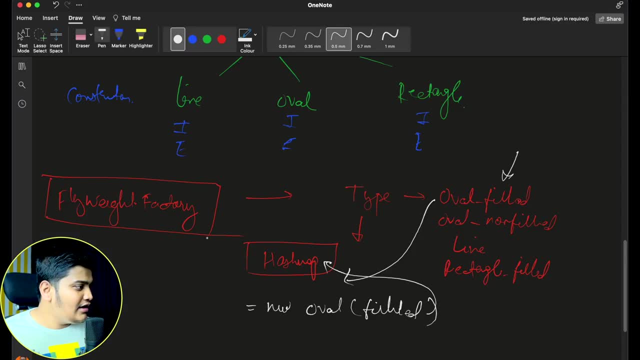 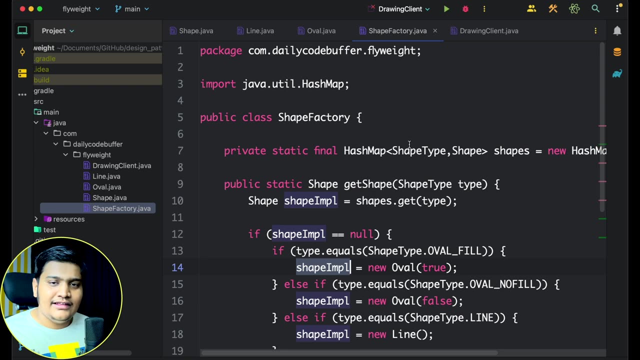 see that. So we have the shapes here already now. as you can see that we have discussed about the flyway factory. here also we have used the flyway factory, that is, the shape factory, and this shape factory will identify the different objects based on the intrinsic values and 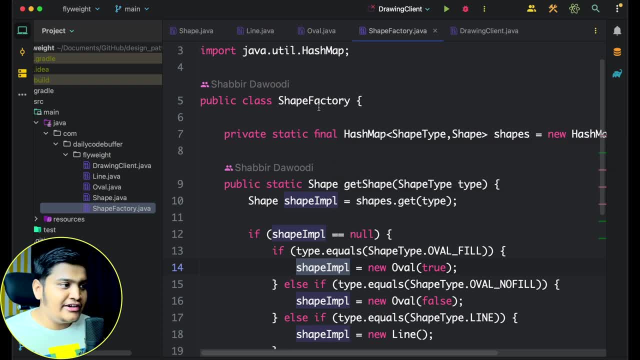 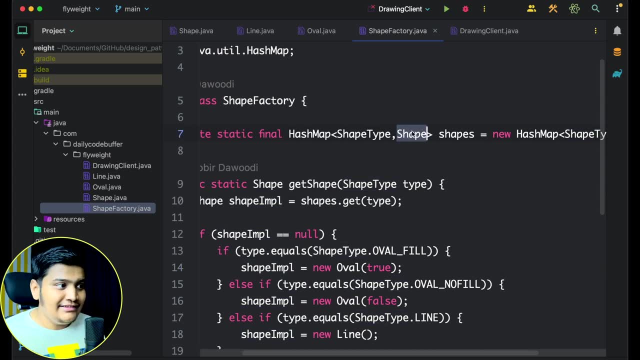 it will return the object if it's available. So here within the shape factory, you can see that we have the hash map of type, shape type and shape. okay, Shape is the interface that we have defined, that what type of shape it is. and shape type we have defined as the enum. 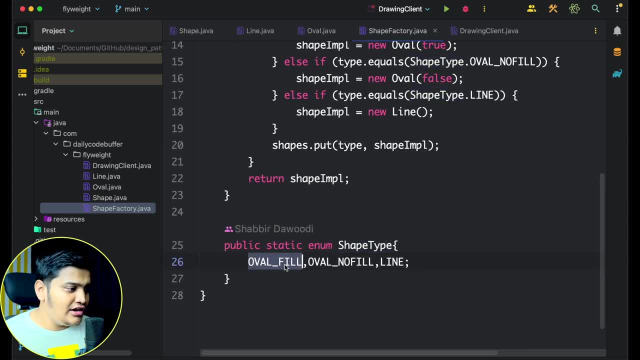 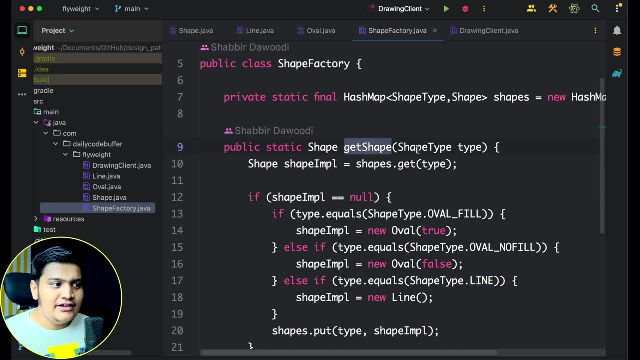 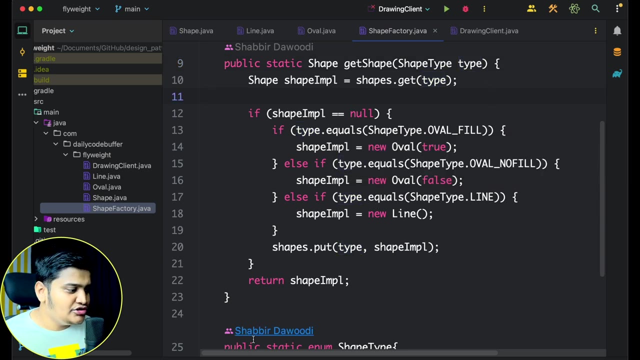 here you can see that what type of shape type it is: it's ovalfill, ovalfill, no fill line whatever we want to create accordingly. okay, and now with the get shape method, you have to pass the shape type and based on that, the object will be created, and that object will be available within the hash map. Suppose here let's take: 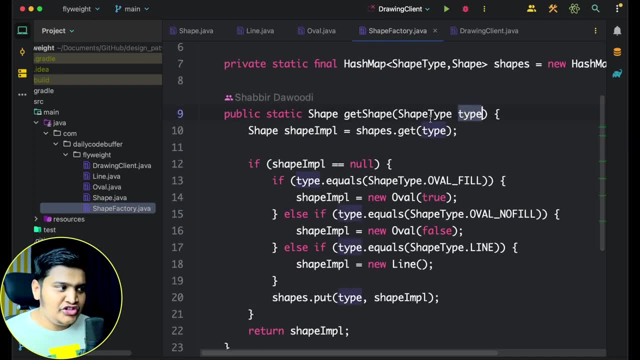 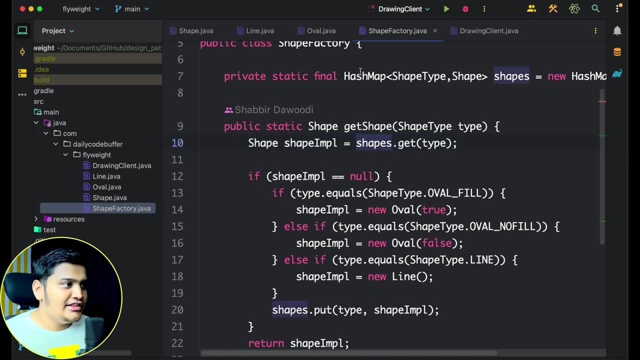 the example of ovalfill. know, we will get the ovalfill here as a shape type and we will here check within the shape implementation that shapes dot get. so within this hash map we will do: shapes dot get ovalfill. Oval fill will not be available because the object is only just created, so we will get. 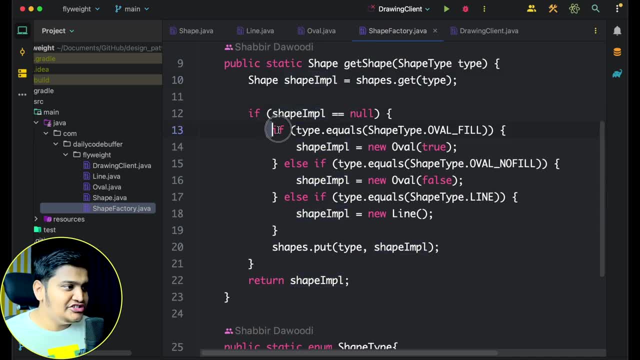 null here. and if we are getting null here, what we will do is we will check what is the shape type. if it's oval, fill, what we will do is we will create a new oval with true. if it's no fill, we will create new oval with false. if line, we will just create line and 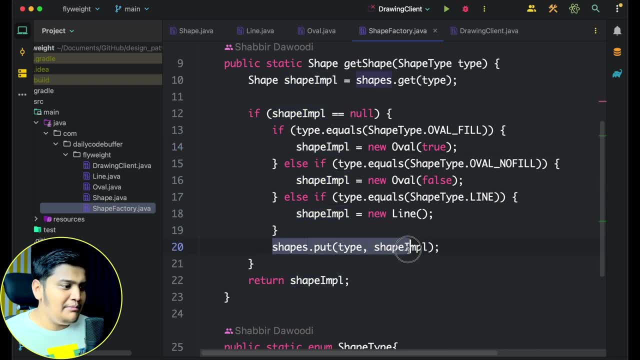 whatever the object is created, we will put that object within the map and we will return the object. so you can see that only once that object is created with the intrinsic values and that object will be available, always within the hash map and from that hash map we will.